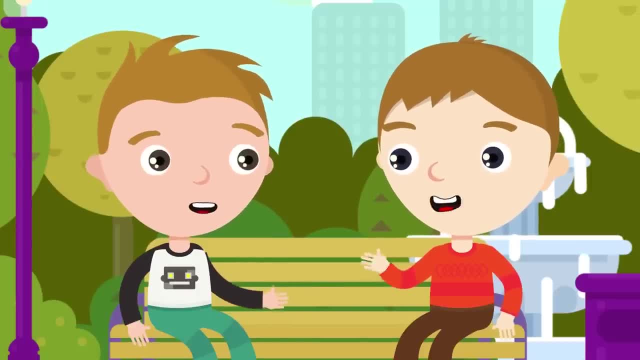 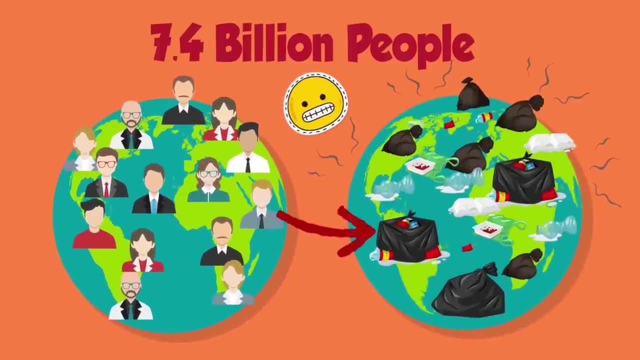 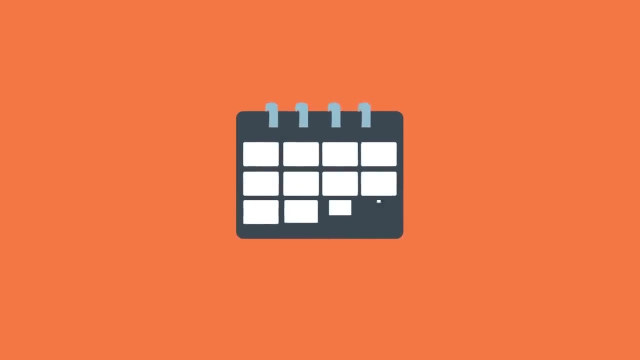 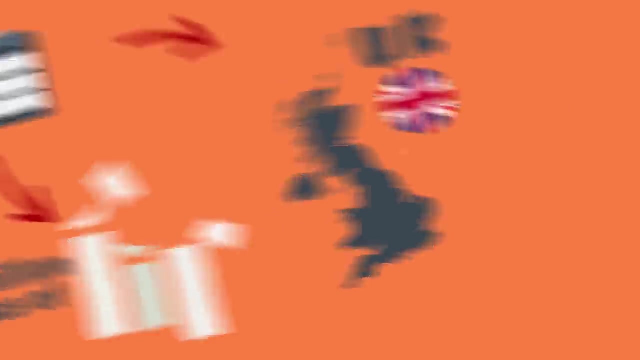 No Well, last year there were 7.4 billion people. Imagine if everyone threw away all their rubbish, The planet would be awful. Every year, 12.5 million tons of paper and cardboard are used just in the UK And it takes 24 trees to make just one ton of waste. 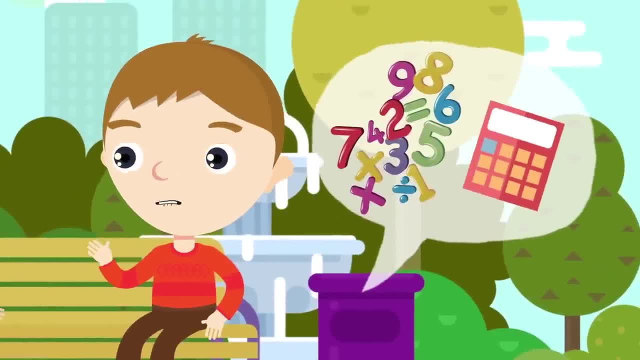 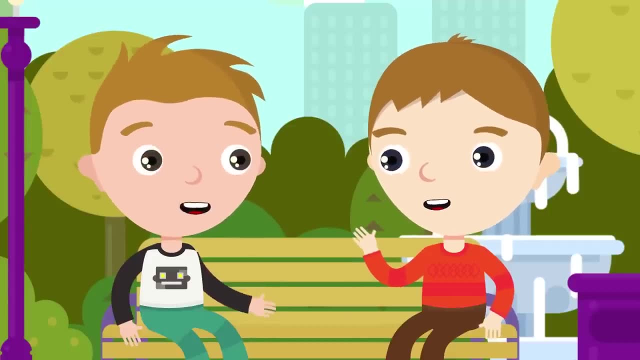 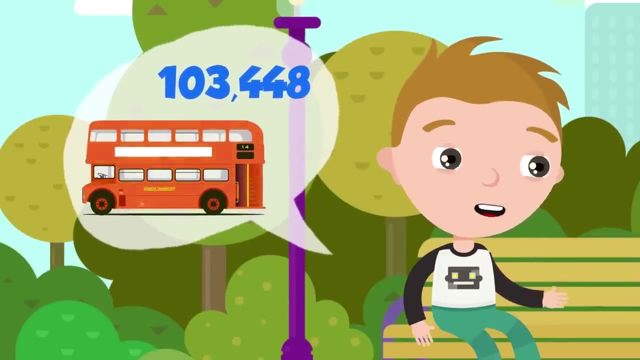 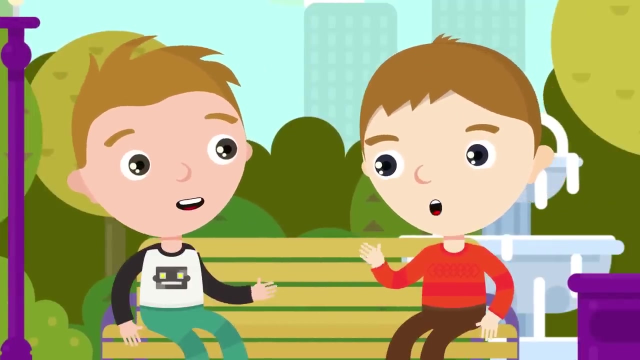 But we have a newspaper. Try multiplying all those numbers, James. Well, by my calculations that will mean that there will be enough paper to fill approximately 103,448 double-decker buses. Really, You just calculated that in your head. Just reducing, reusing and recycling some brain parts. we are at the end of our study. 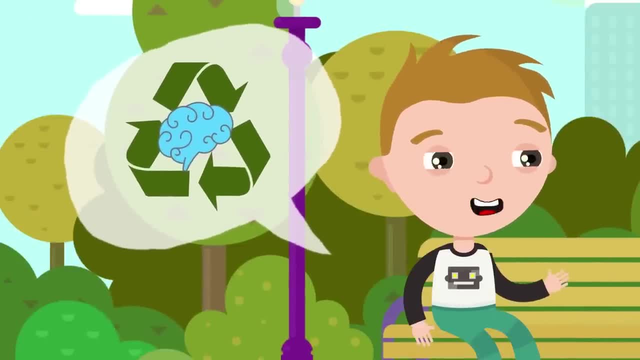 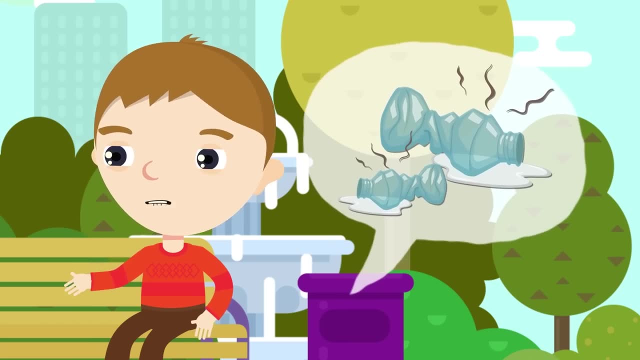 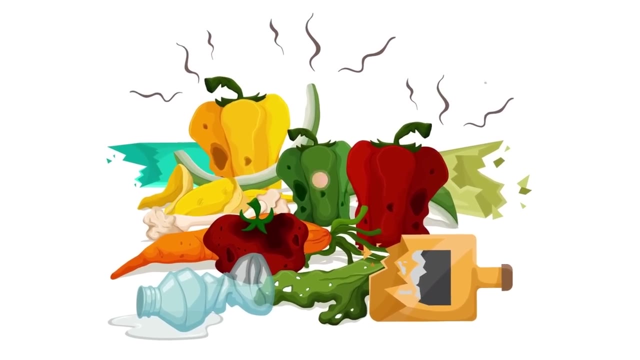 Just reducing, reusing and recycling some brain parts. Really You just calculated that in your head: Just reducing, reusing and recycling some brain parts- funny. also, did you know that some plastic can take over 500 years to decompose? what does decompose mean? it means to break down or rot, so you mean a. 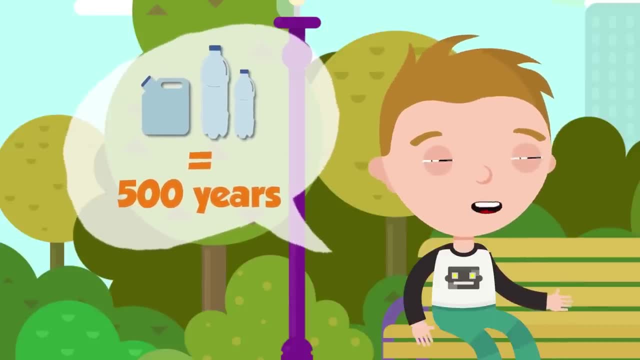 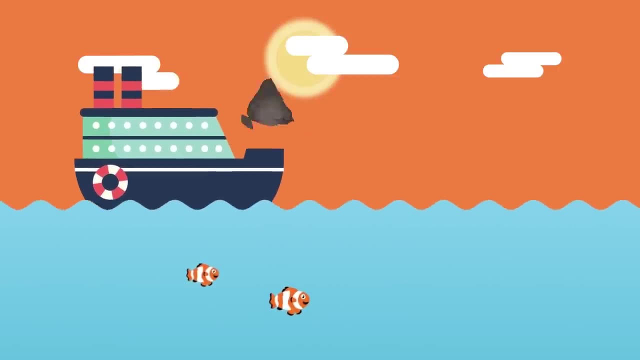 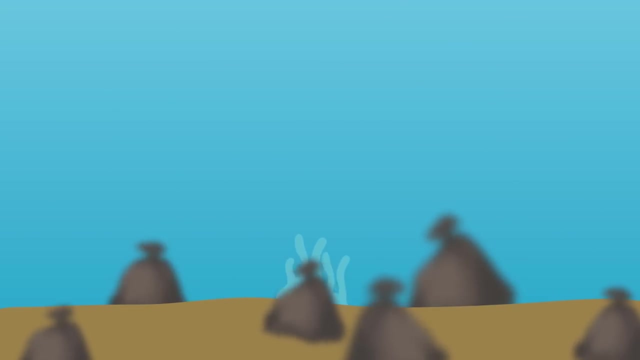 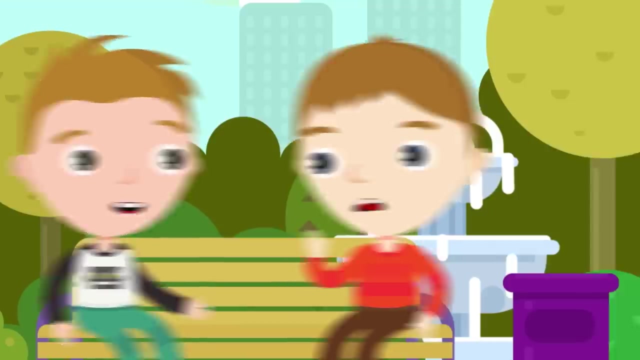 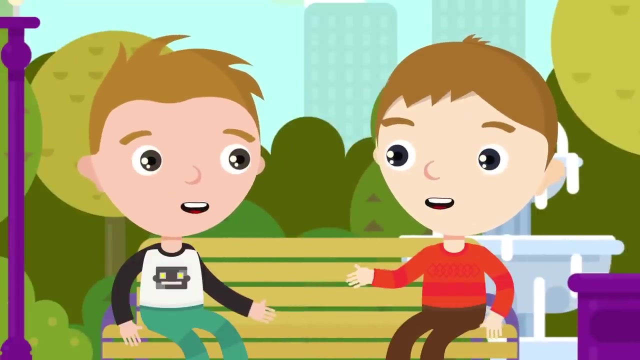 piece of plastic can be around for 500 years exactly. and even worse than that, plastic bags and rubbish thrown into oceans around the world kill more than 1 million marine mammals, fish and sea creatures every year. oh no, poor little creatures. yet another amazing fact. do you know the polystyrene cups that you drink out of and then throw away? yes, like at parties. yes, well, if you. 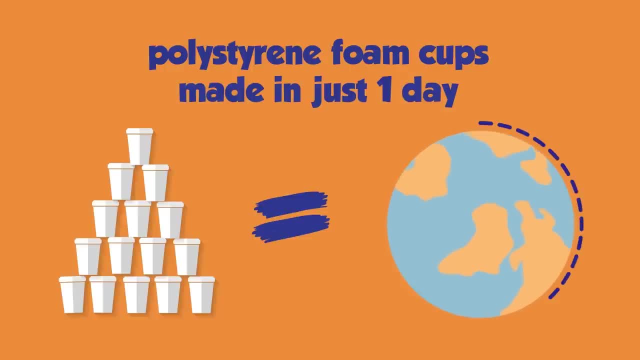 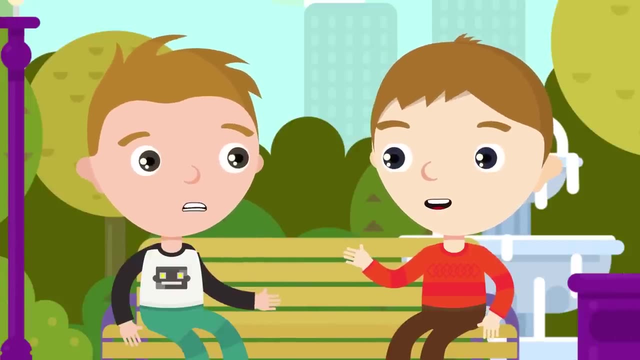 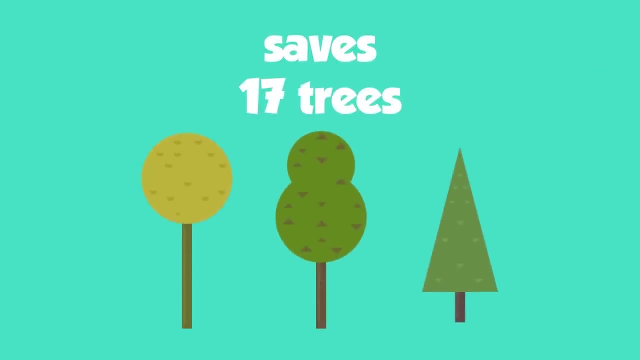 lined up all the polystyrene foam cups made in just one day. they would circle the earth that many, ever, every day. why don't people use reusable cups? now you're getting the idea. reduce, reuse, recycle. recycling: just one ton of paper saves 17 trees, 6000 gallons of water and produces 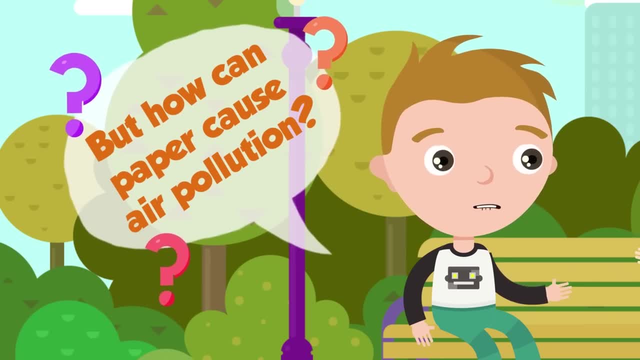 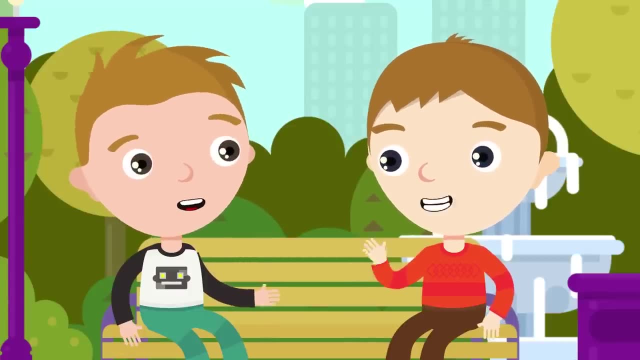 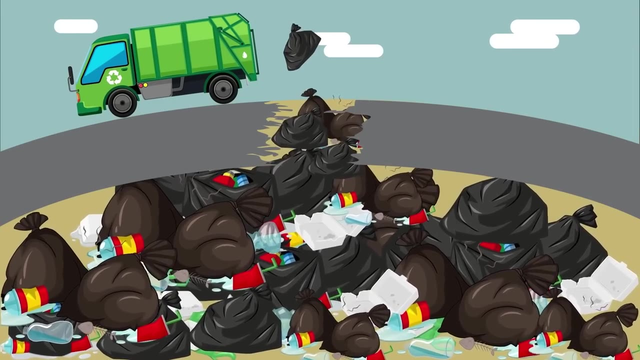 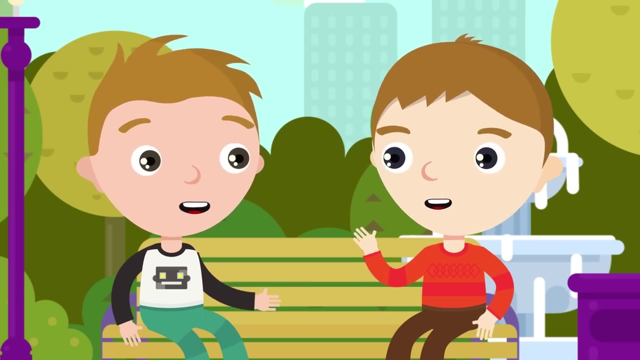 less air pollution. but how can paper cost air pollution? if rubbish, including paper, is not recycled, it may go to another landfill site. what's a landfill site? a landfill site is a place where rubbish is dumped and then buried. oh yes, so how does a pile of buried rubbish cause air? 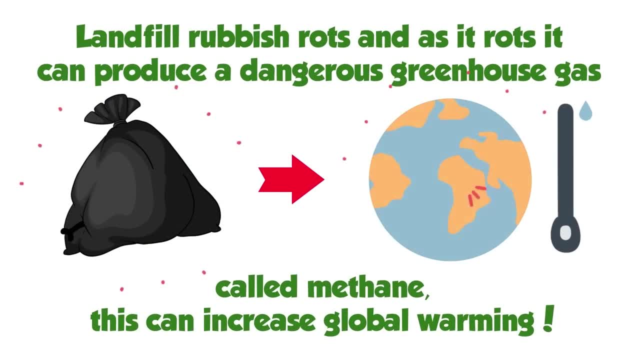 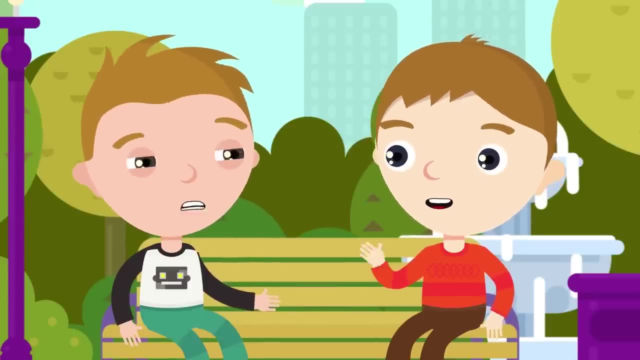 pollution. well, landfill rubbish rot and as it rot it can produce a dangerous greenhouse gas called methane. this can increase global warming. this is also interesting. I never realized how important it is to recycle. yes, it is so important if we want to help the planet and our environment, recycling just one glass. 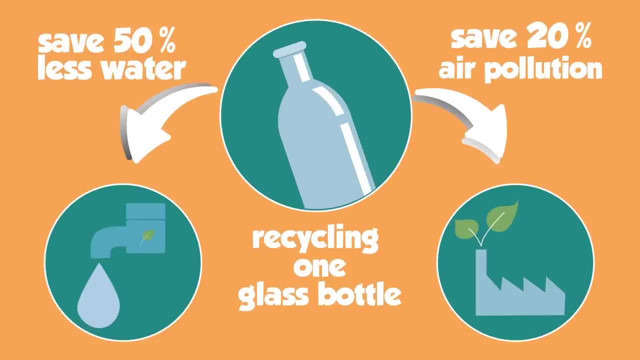 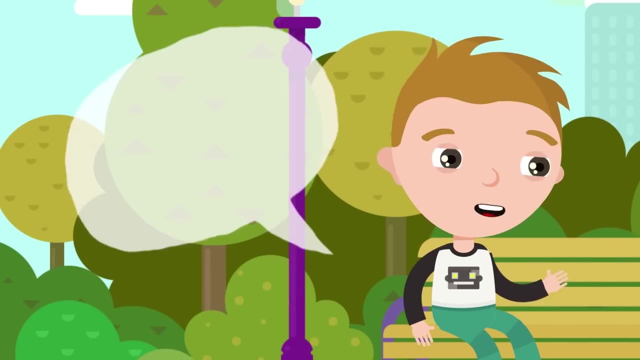 bottle can save 20% air pollution and 50% less water than making the bottle from scratch. what you can recycle glass too- oh yes. recycling plastic waste can save 20% air pollution and 50% less water than making the bottle from scrap. what you can recycle- glass too- oh yes, recycling plastic is. 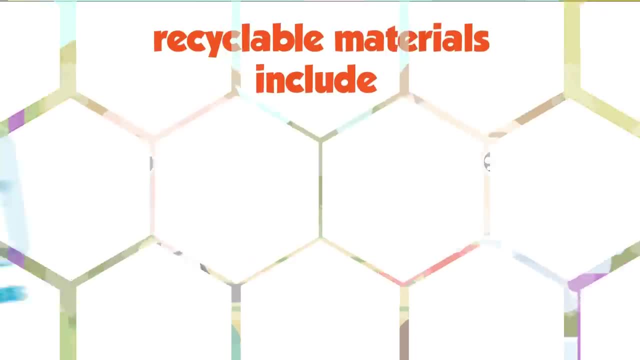 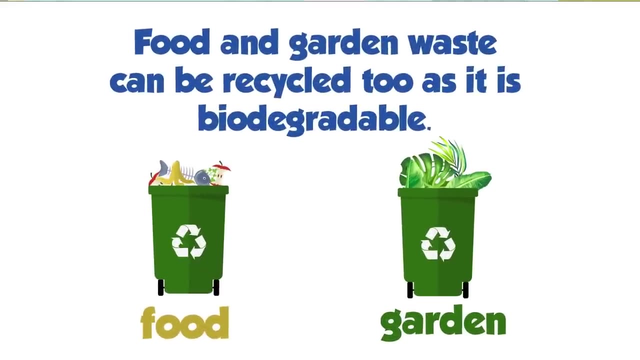 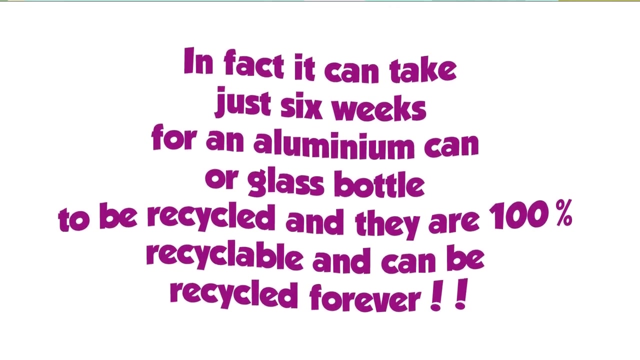 recyclable Materials include glass, paper, metal, plastic fabrics and electronics. Food and garden waste can be recycled too, as it is biodegradable. In fact, it can take just six weeks for an aluminium can or glass bottle to be recycled, and. 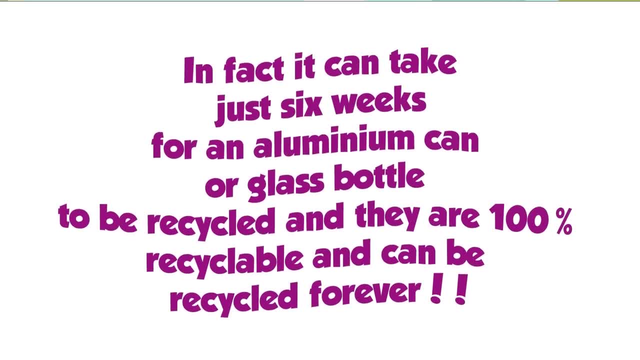 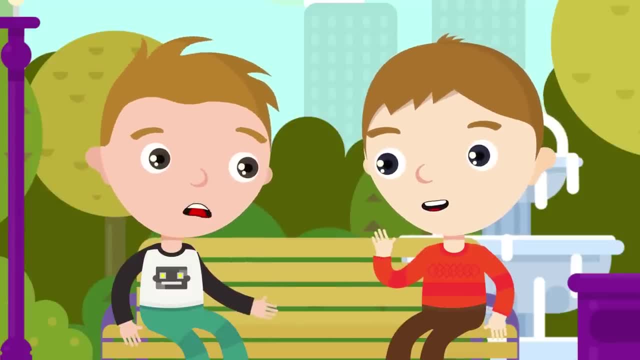 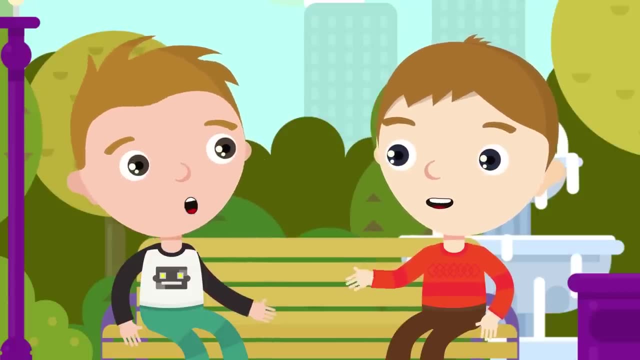 they are 100% recyclable and can be recycled forever. Simply amazing. I can't believe that I've just gone to throw my rubbish away. Recycling is so important for us, the planet, animals and the environment. I'll never see rubbish in the same way. 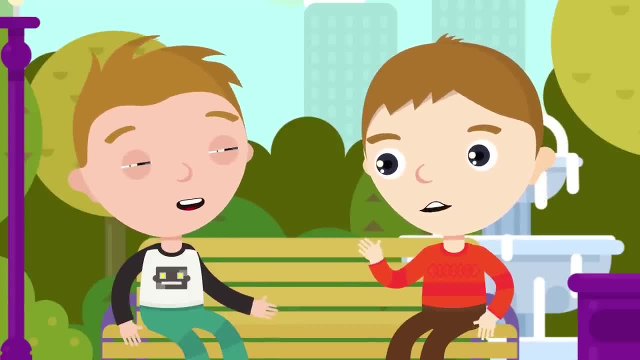 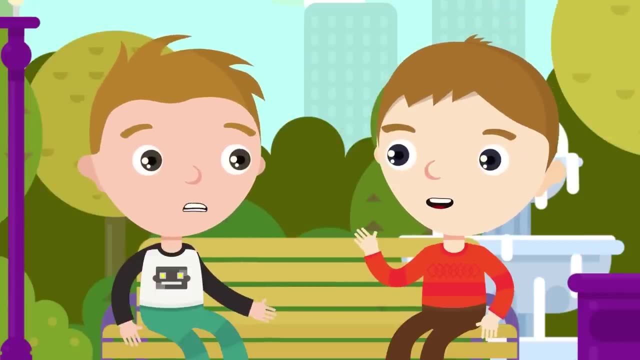 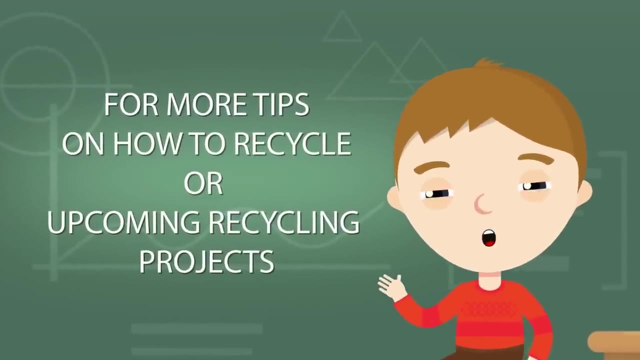 again. Rubbish really can be amazing, as long as we all remember to reduce, reuse, recycle. Thanks, Aaron, I'm off to do some recycling of my own. Good job, James. For more tips on how to recycle, or upcoming recycling projects, why not? 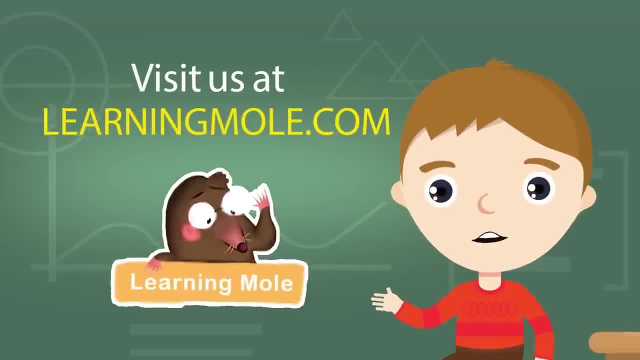 subscribe or pop over and visit us at wwwlearningmallcom.